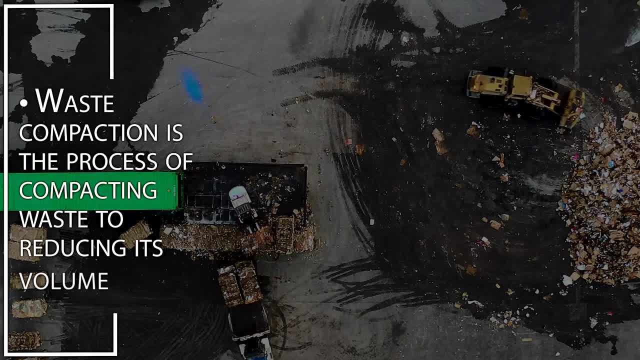 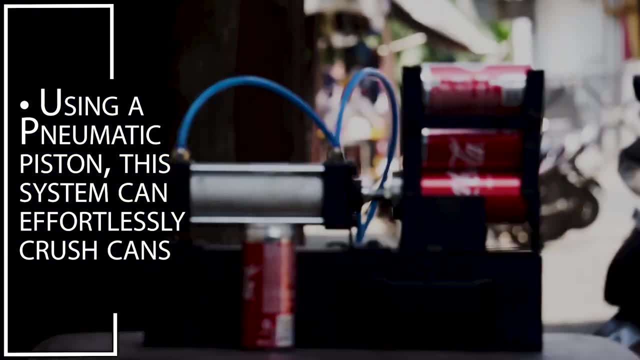 Pneumatic Can Crusher. Waist compaction is a process of compacting waste to reducing its volume. Using a pneumatic piston, the system can effortlessly crush cans. This system can reduce a can to one-third of its size at the touch of a button. 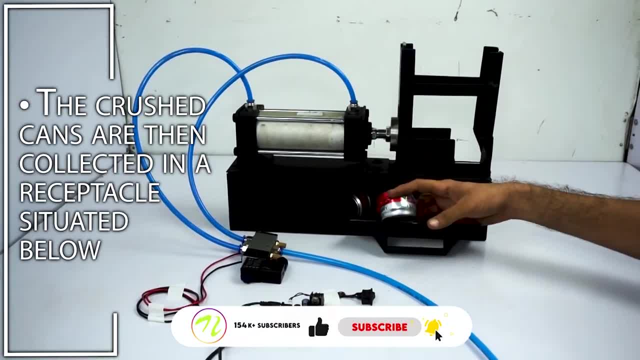 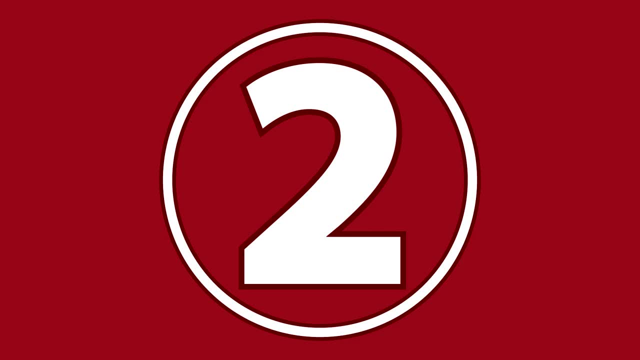 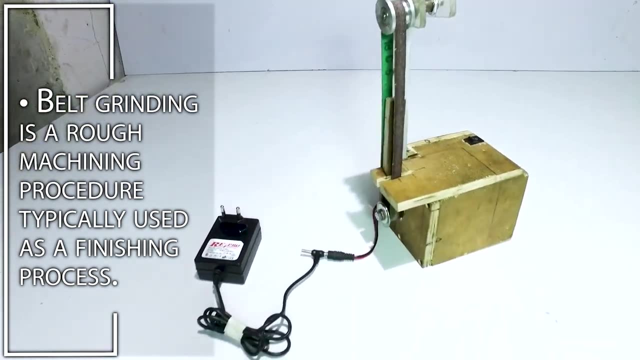 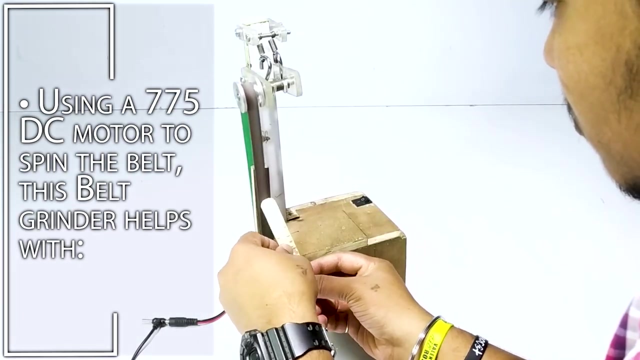 The crushed cans are then collected in a receptacle situated below Mini Belt Grinder. Belt grinding is a rough machining procedure typically used as a finishing process. A belt covered in abrasive material is kept running over the surface to be processed Using a 775 DC motor to spin the belt. this belt grinder helps with 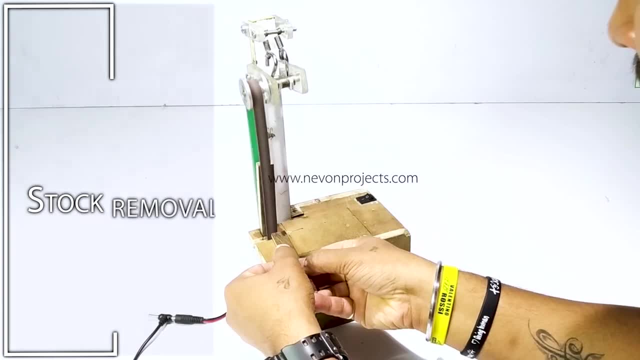 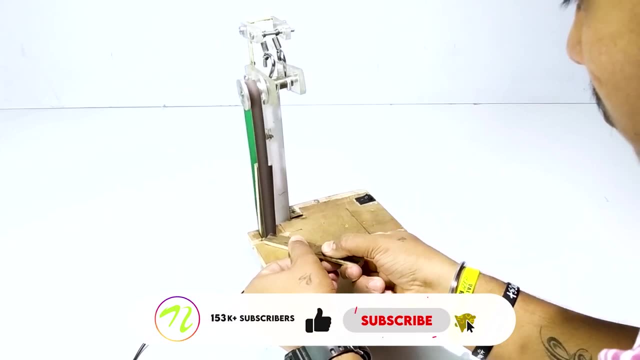 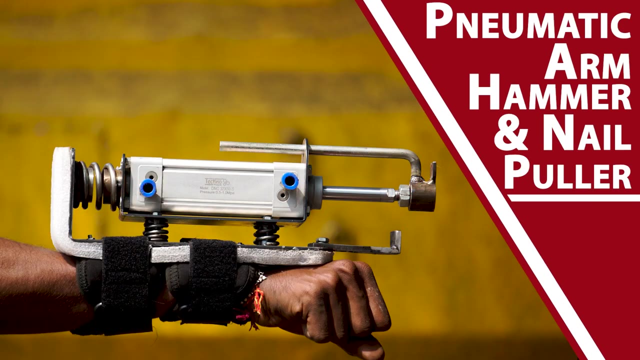 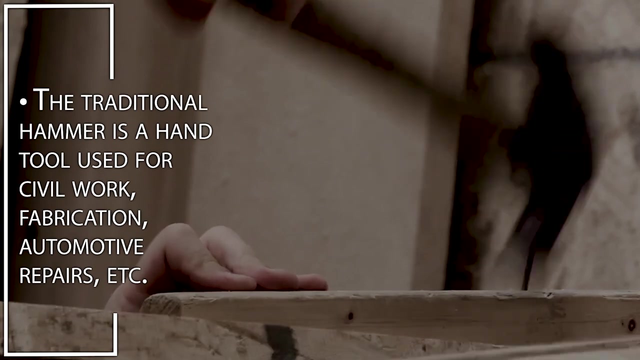 polishing, burr removal, cleaning, stock removal and radiusing. Pneumatic Arm Hammer and Nail Puller. The traditional hammer is a hand tool used for civil work, fabrication, automotive repairs, etc. This arm hammer improves on the existing technology by 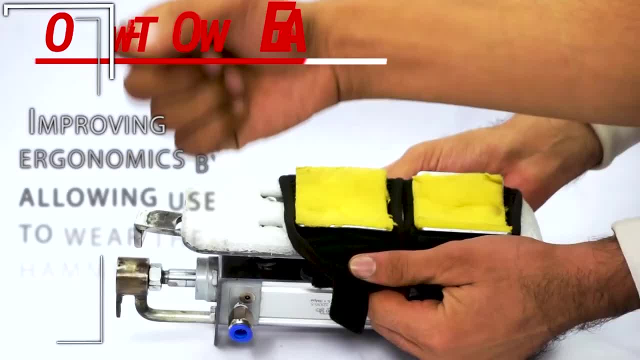 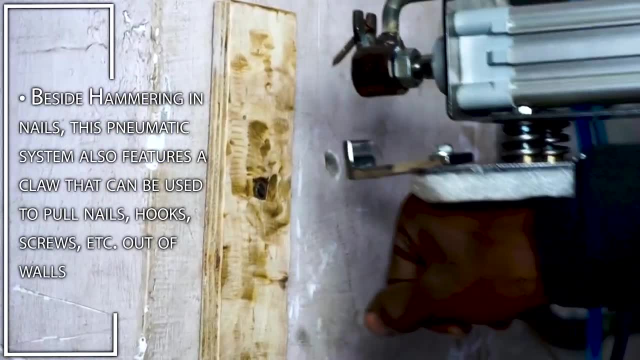 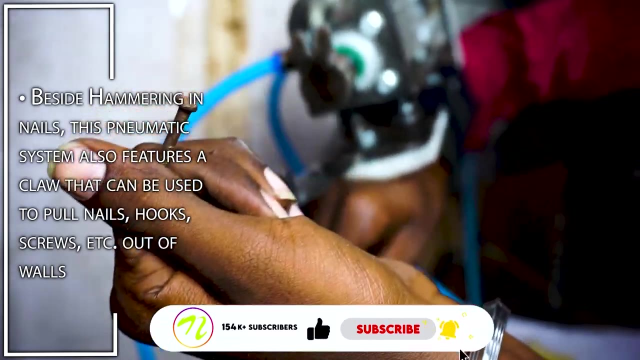 Using pneumatics to improve efficiency of hammering, Improving ergonomics by allowing user to wear the hammer on their hand. Besides hammering in nails, this pneumatic system also features a claw that can be used to pull the nails, hooks, screws, etc. out of the walls. 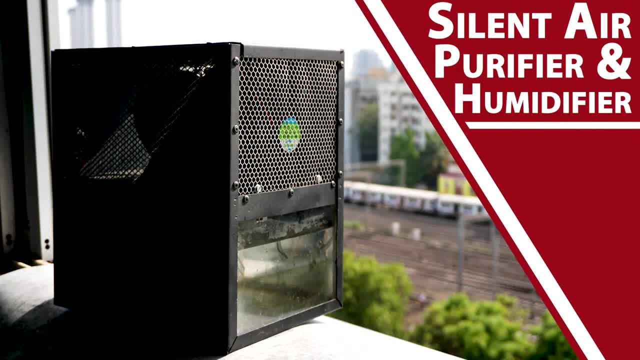 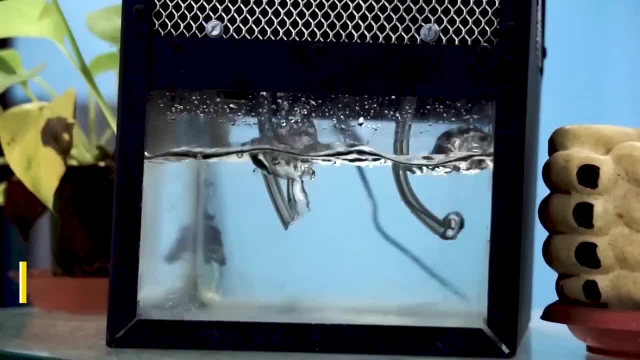 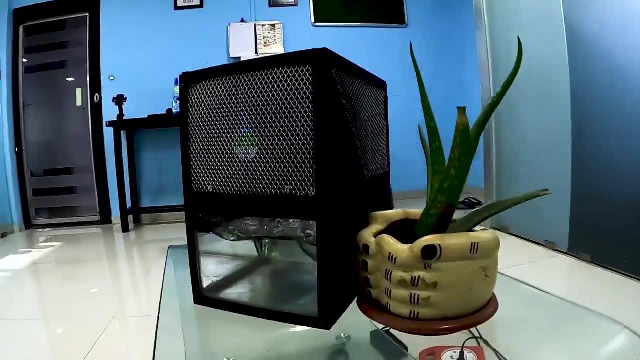 Silent Air Purifier and Humidifier. In recent years, pollution levels across the globe have skyrocketed, causing the AQI to plummet. This silent air purifier uses water to filter out pollutants, thereby eliminating the need for expensive filters, Along with being silent. 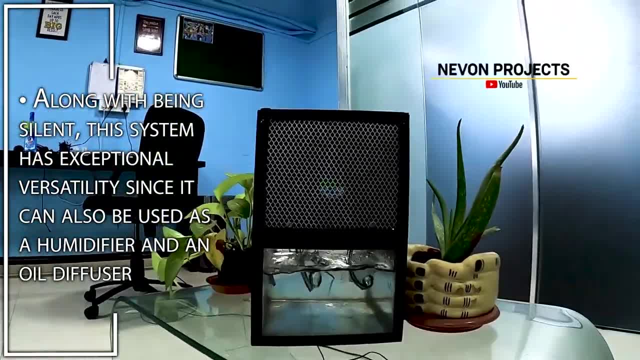 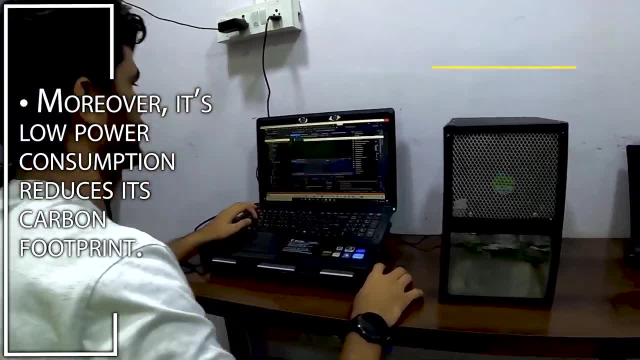 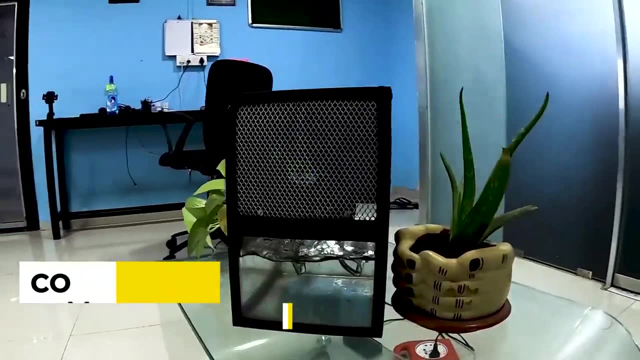 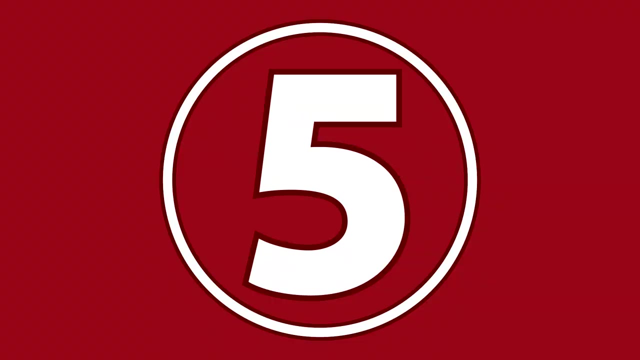 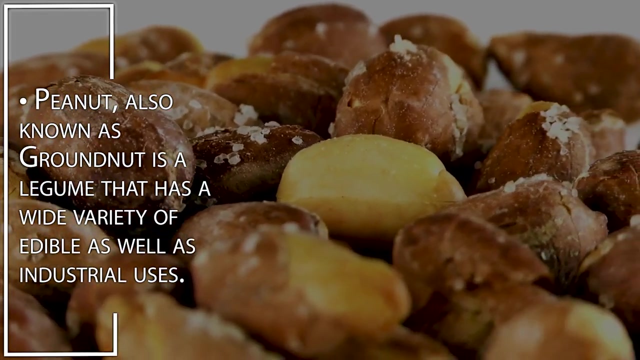 the system has exceptional versatility, since it can also be used as a humidifier and an oil diffuser. Moreover, its low power consumption reduces its carbon footprint. Groundnut and Peanut Shelling. Peanut, also known as groundnut, is a legume that has a wide variety of edible as well as industrial uses. 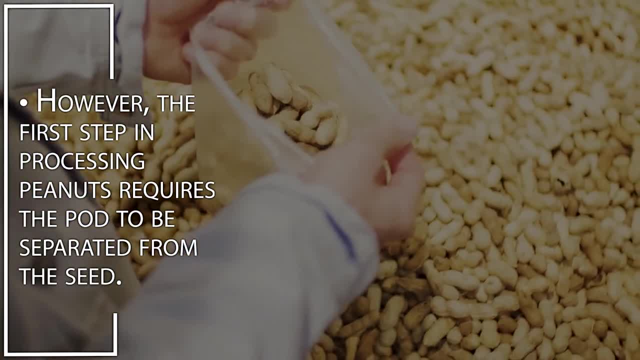 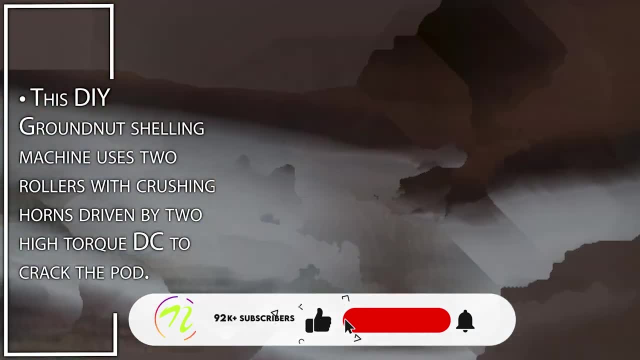 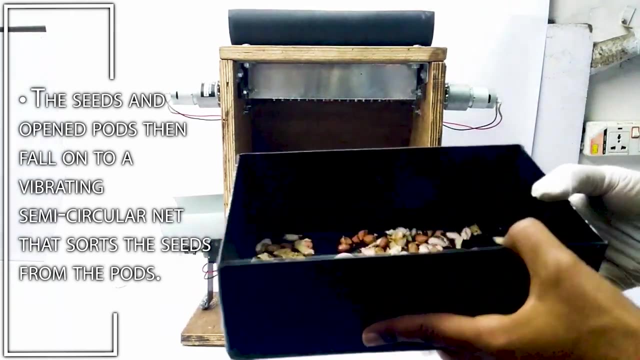 However, the first step in processing peanut requires the pod to be separated from the seed. This DIY groundnut shelling machine uses two rollers with crushing horns driven by two high-speed DC motors to crack the pod. The seeds and open pods then fall onto a vibrating semi-circular net that sorts the seed from the pods. 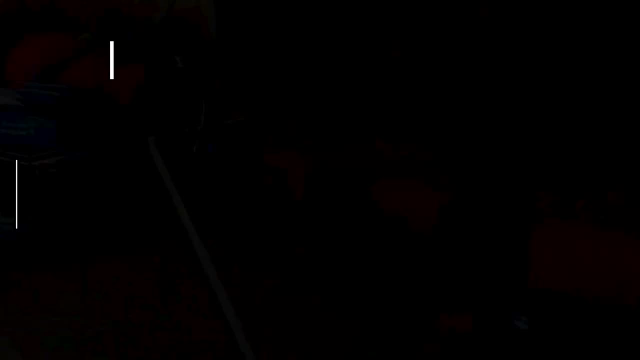 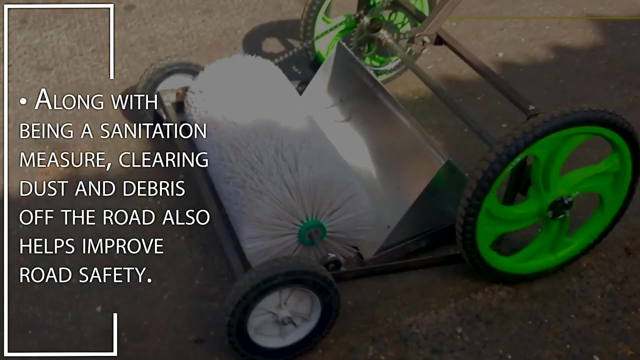 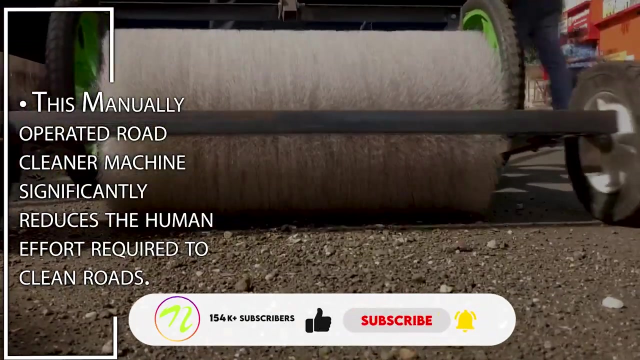 Manually operated road and floor cleaning machine. Along with being a sanitation measure, clearing dust and debris off the road also helps improve road safety. This manually operated road cleaner machine significantly reduces the human effort required to clean roads. Along with being eco-friendly, the system is extremely user-friendly and can be operated by anyone. 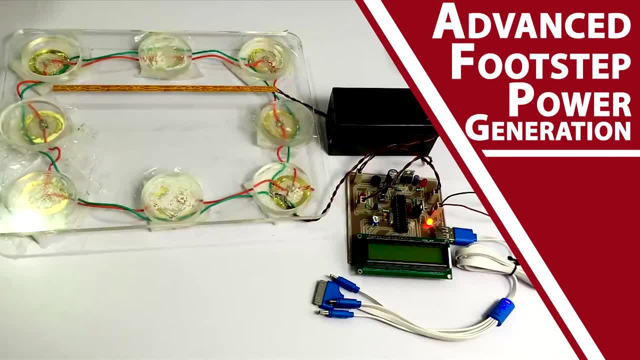 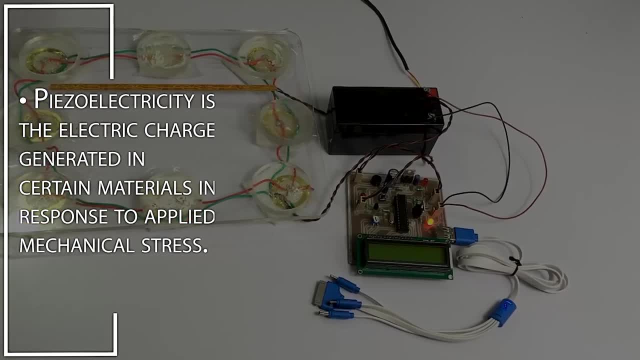 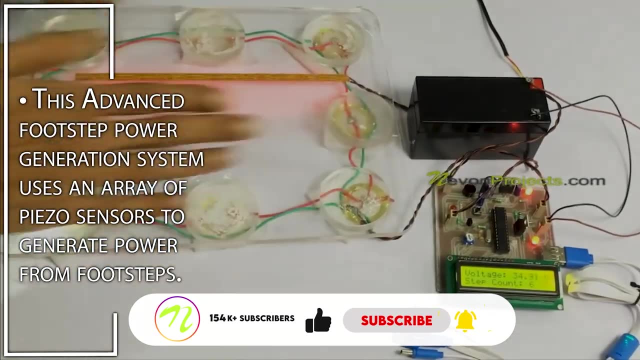 Advanced Footstep Power Generation. Piezoelectricity is the electric charge generated in certain materials in response to applied mechanical stress. This advanced footstep power generation system uses an array of piezo sensors to generate power from footsteps. The voltage generated from piezo sensors is used to charge a battery. 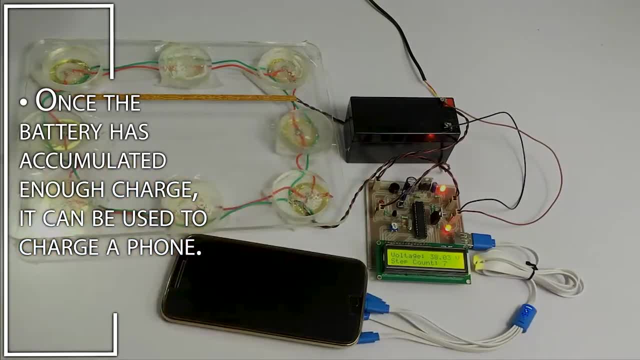 Once the battery has accumulated enough charge, it can be used to charge a phone. This system also features a USB port that can be used to charge a phone. This system also features a USB port that can be used to charge a phone. This system also features a USB port that can be used to charge a phone. 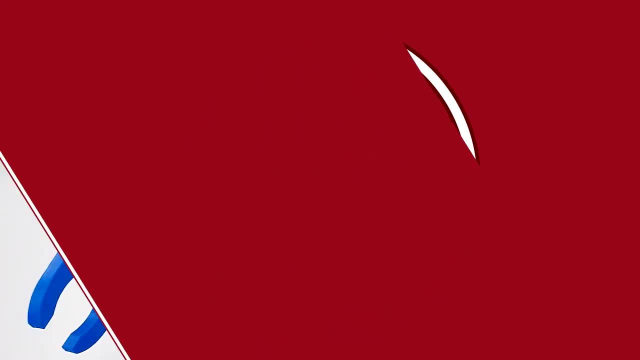 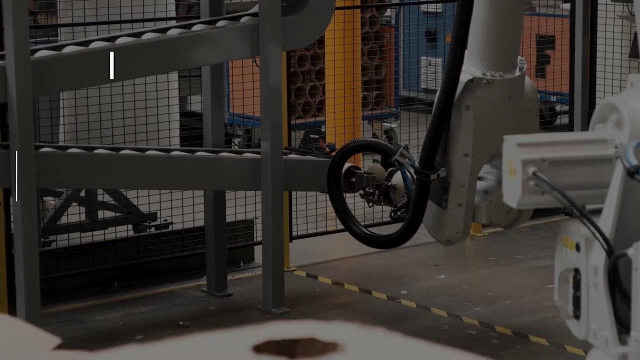 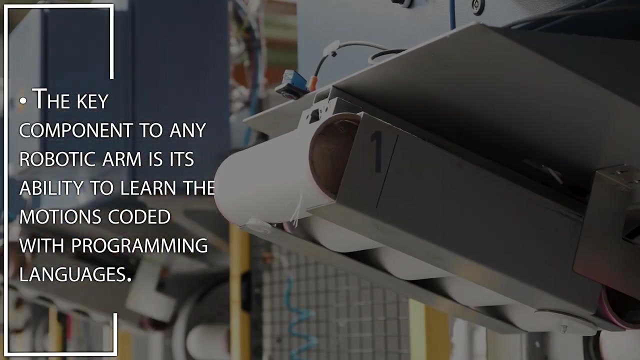 smart watch, headphones, etc. Android-controlled Robotic Arm. Robotic arms have a broad range of applications in industrial automations. The key component to any robotic arm is its ability to learn the motions coded with programming languages. This Arduino-based robotic arm can be programmed via smartphone to perform any task desired by the user. 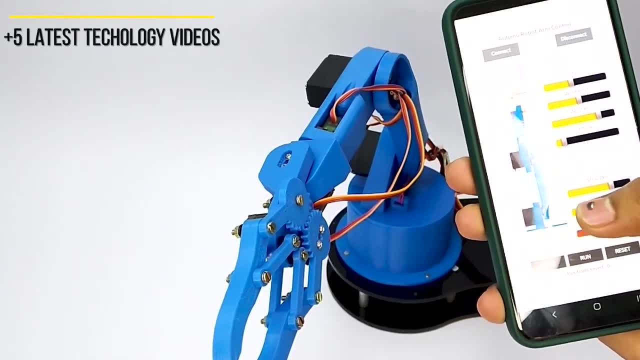 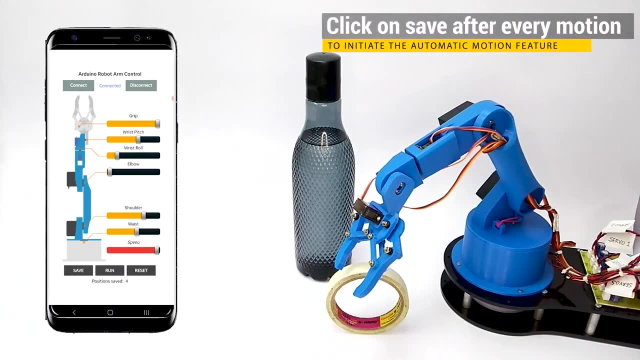 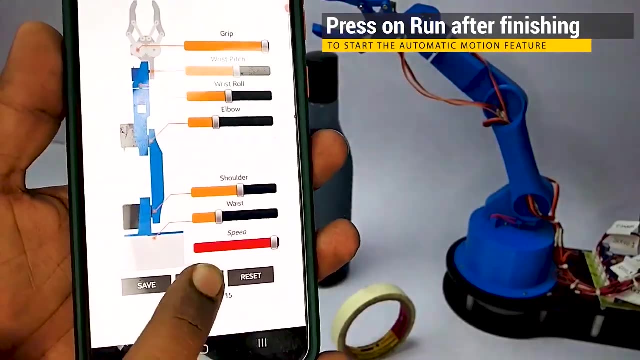 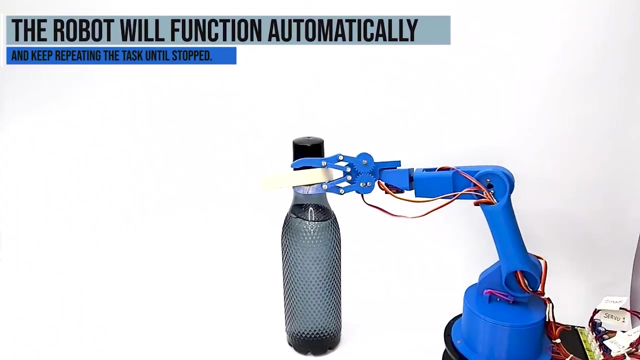 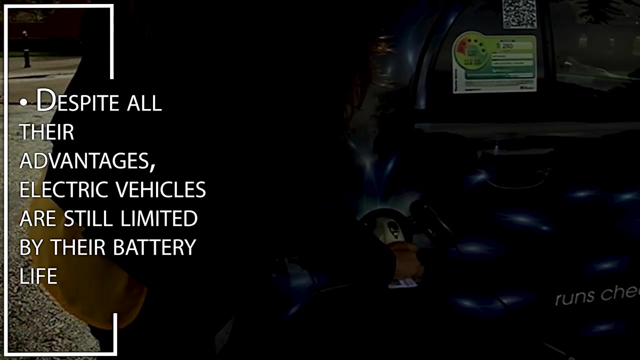 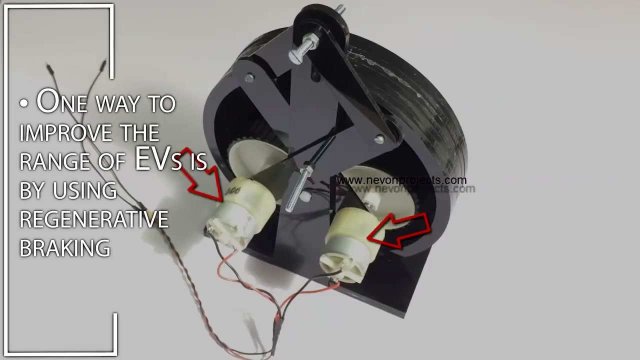 This Arduino-based robotic arm can be programmed via smartphone to perform any task desired by the user. REGENERATIVE BREAKING SYSTEM. Despite all their advantages, electric vehicles are still limited by their battery life. One way to improve the range of EVs is by using regenerative braking. 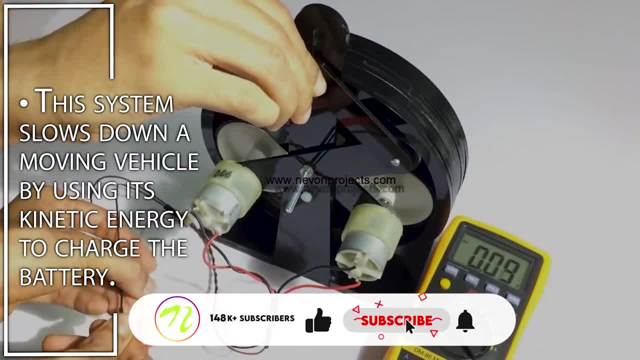 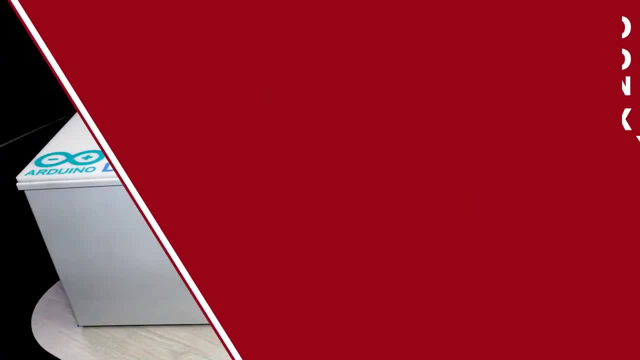 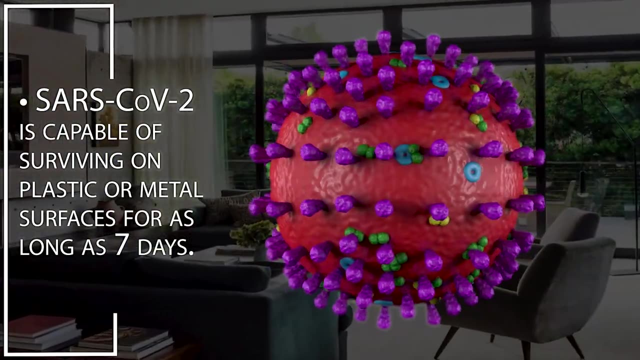 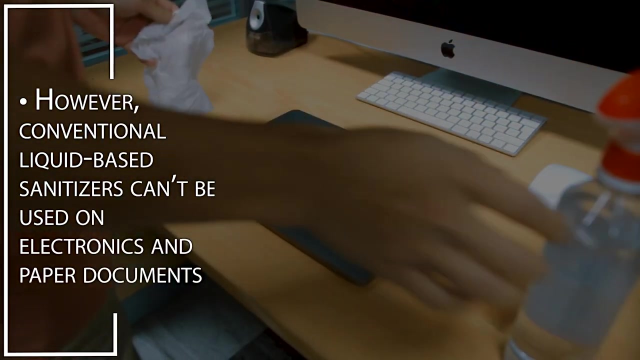 This system slows down a moving vehicle by using its kinetic energy to charge the battery. ARDENO COVID DISINFECTION BOX SARS-CoV-2 is capable of surviving on plastics or metal surfaces for as long as 7 days. However, conventional liquid-based sanitizers can't be used on electronics and paper documents. 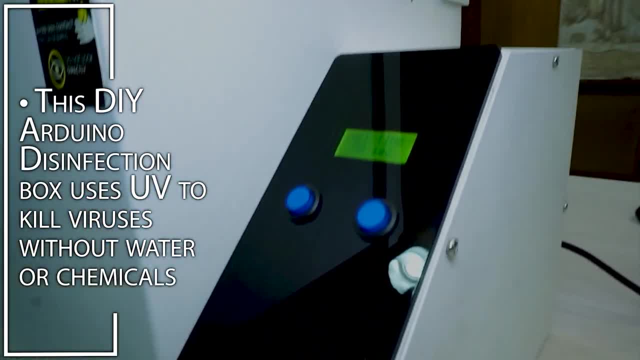 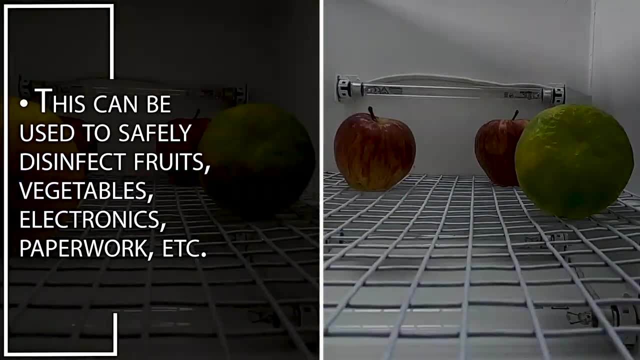 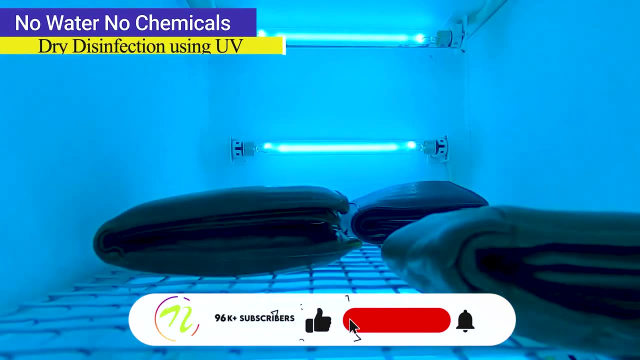 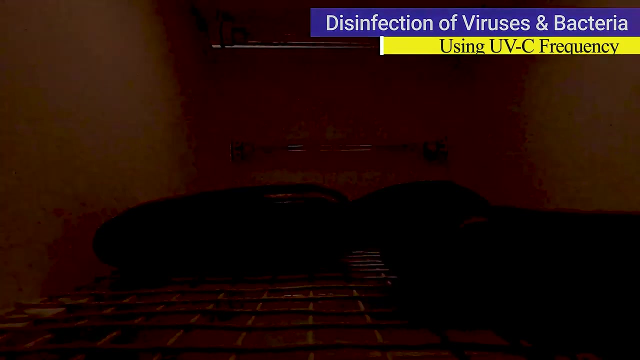 This DIY ARDENO disinfection box uses UV to kill viruses, without water or chemicals. This can be used to safely disinfect fruits, vegetables, electronics, paperworks, etc. This device can be used to protect your car from a car accident and prevent the car from getting damaged. 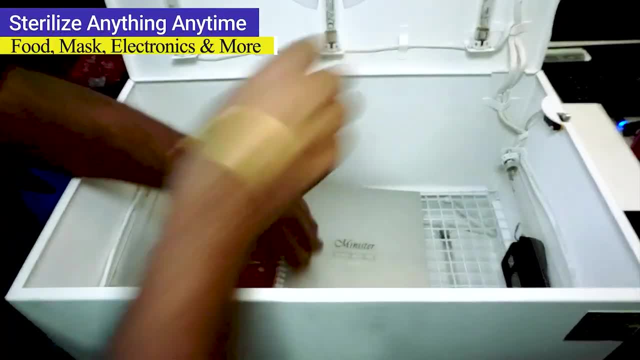 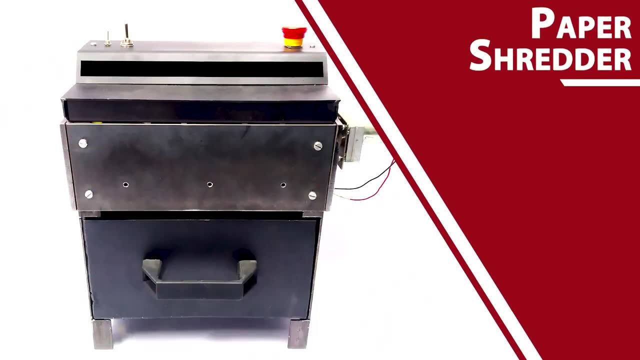 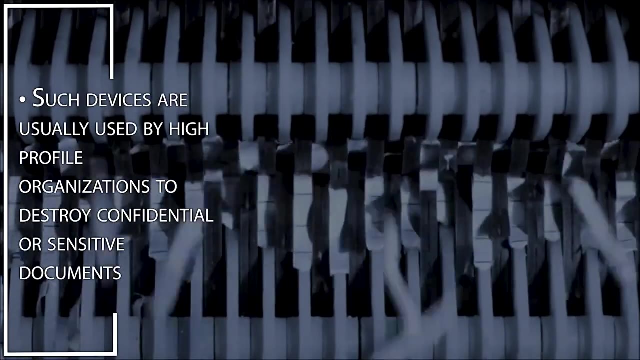 It can also be used to protect your car from potential accidents. PAPER SHREDDER- A paper shredder is a machine used to cut paper into thin strips. Such devices are usually used by high-profile organizations to destroy confidential or sensitive documents. Such devices are usually used by high-profile organizations to destroy confidential or sensitive documents. 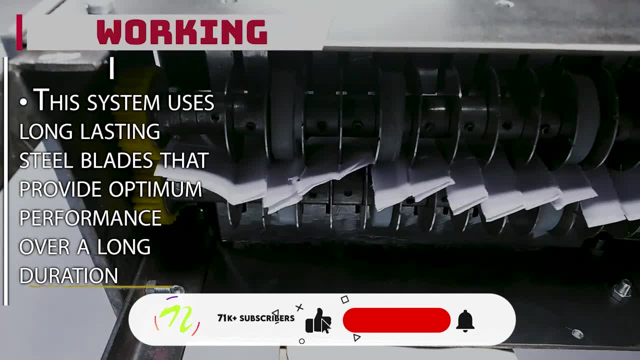 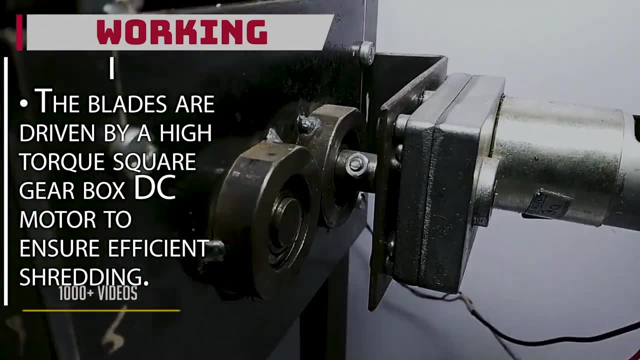 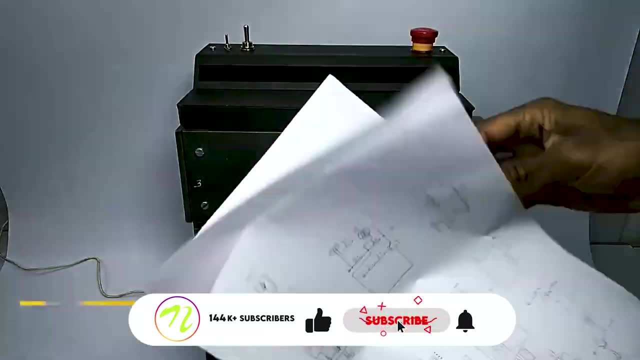 This system uses long-lasting steel blades that provide optimum performance over a long duration. The blades are driven by a high-torque square gearbox DC motor to ensure efficient shredding. Moreover, its compact size makes it very easy to move around. PAPER SHREDDER. 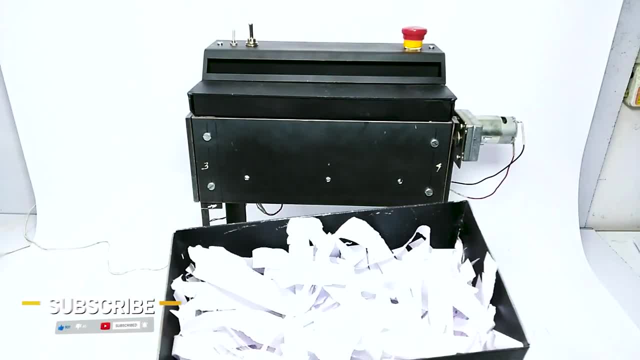